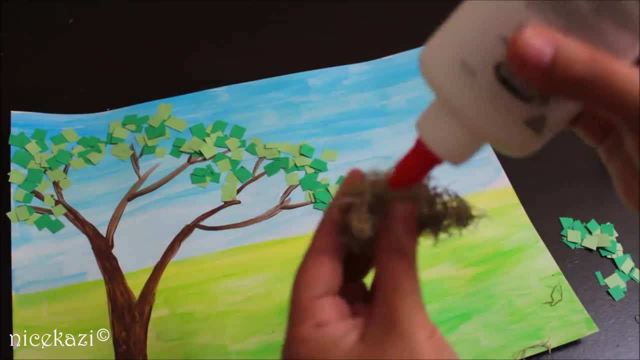 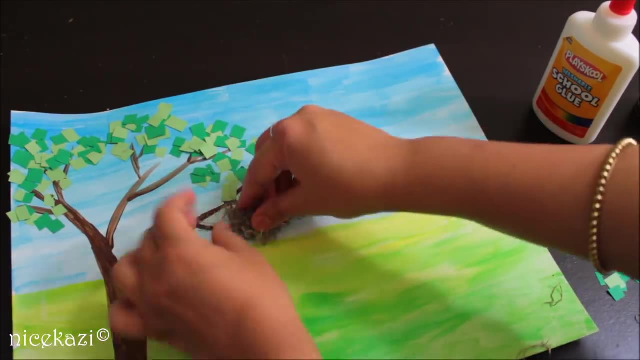 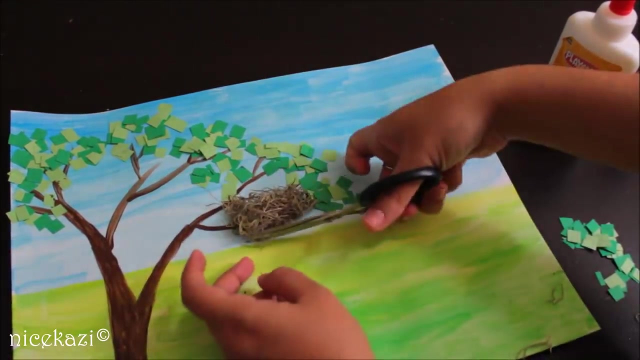 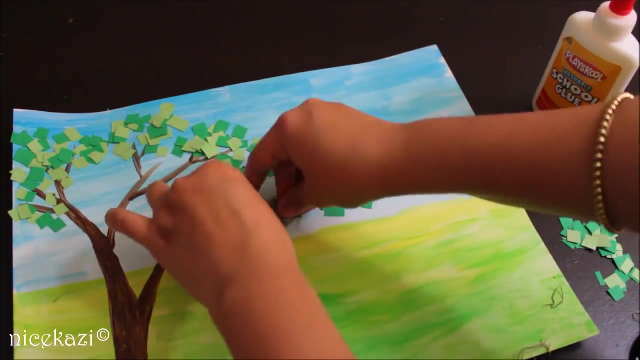 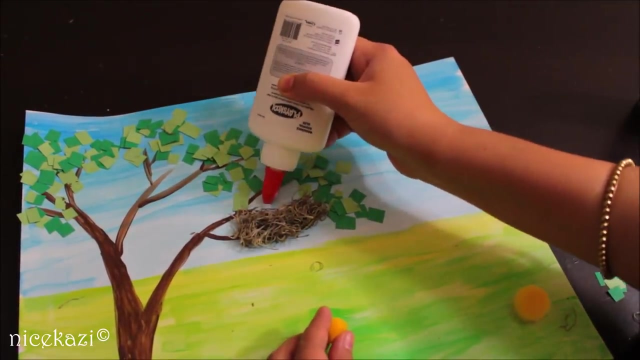 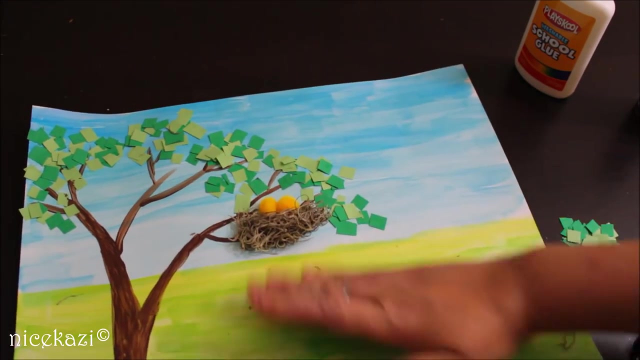 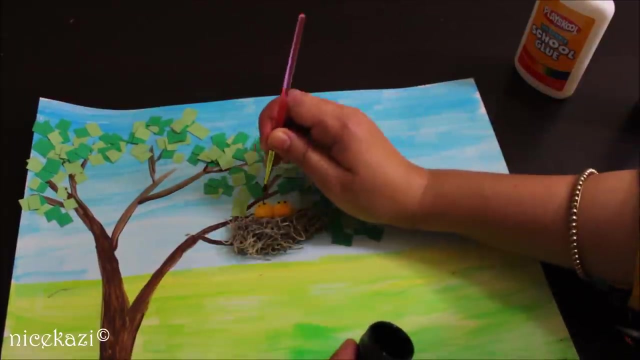 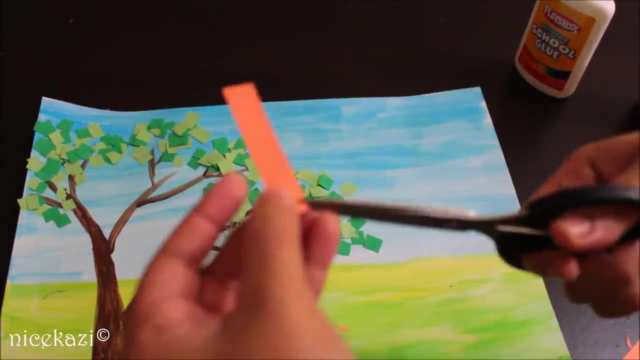 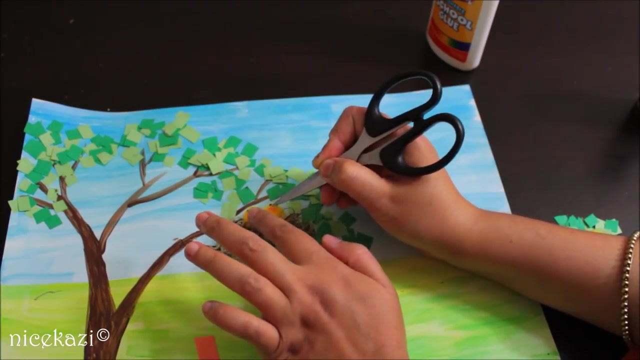 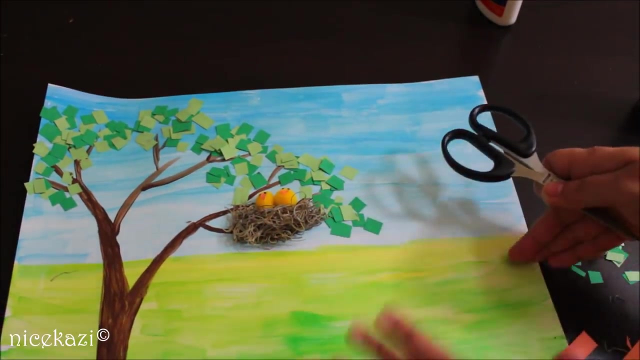 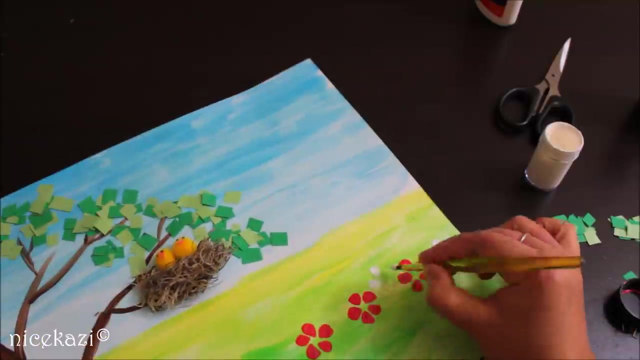 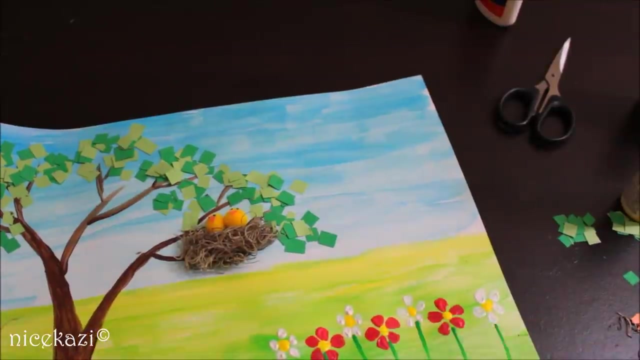 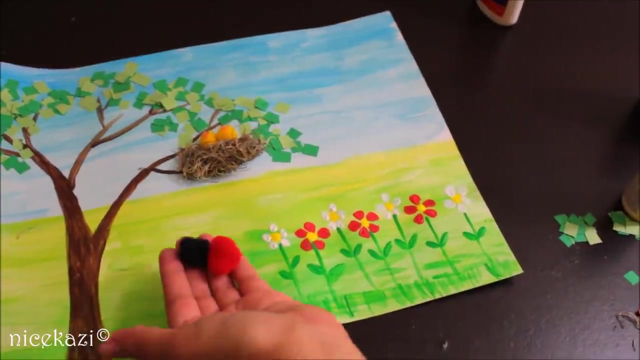 Let's stick the nest with glue. Now, with this pom pom, I am going to make baby birds. For eyes, I used black acrylic color. I used orange construction paper for their beaks. Now let's paint the flowers. Let's make a ladybug with this pom-pom. 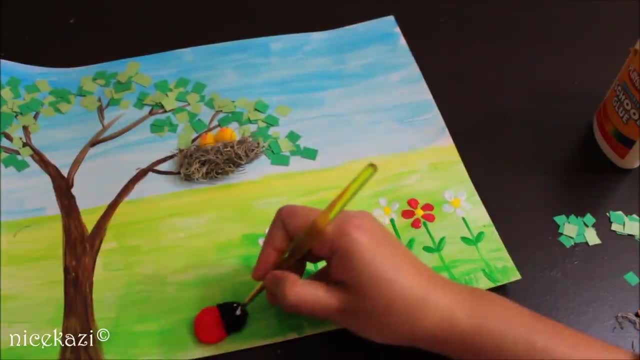 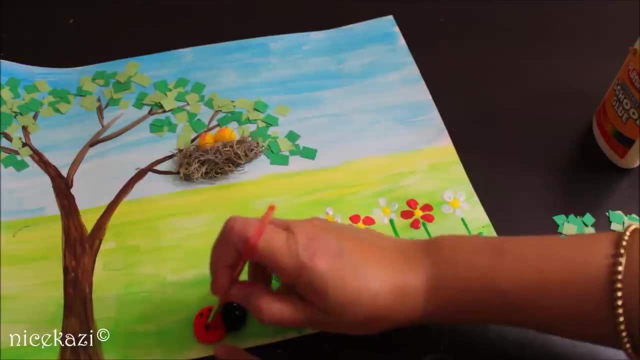 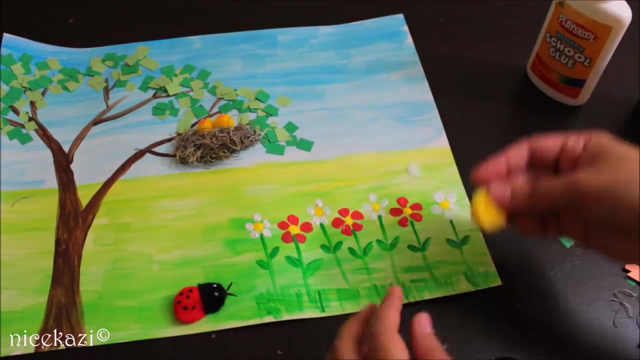 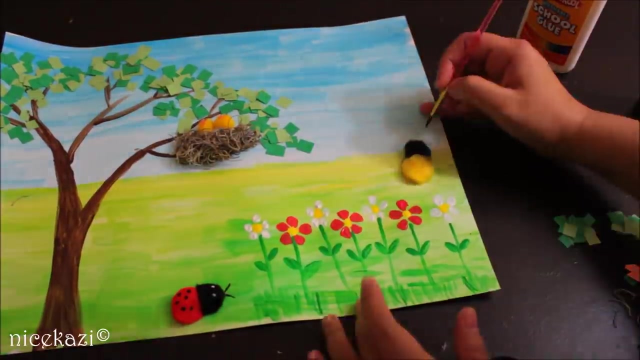 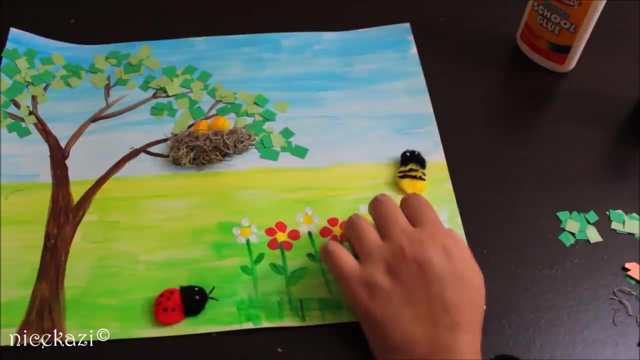 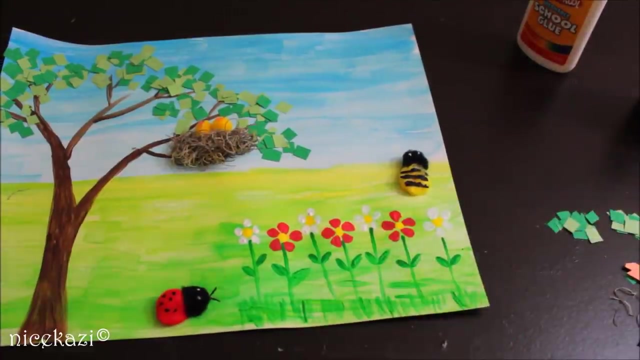 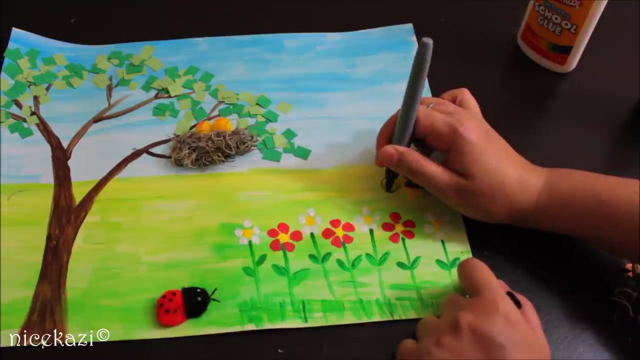 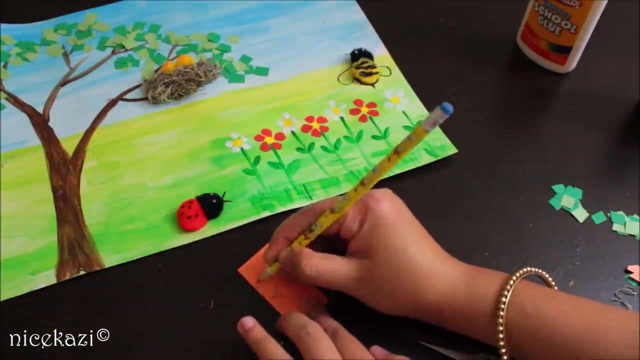 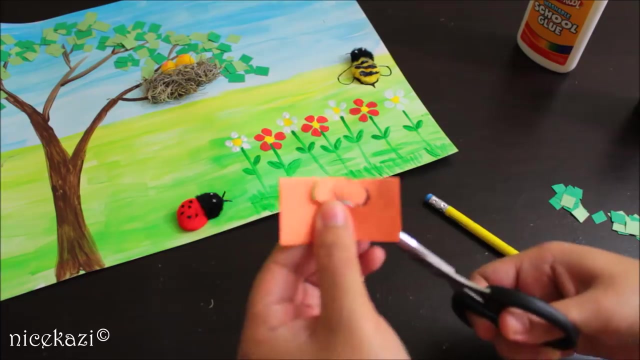 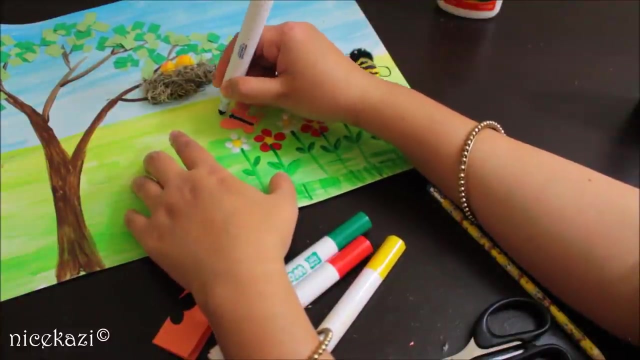 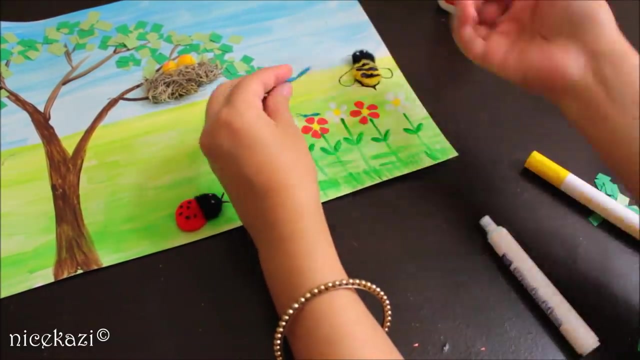 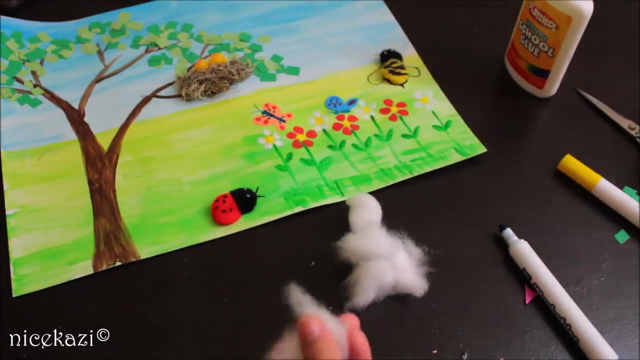 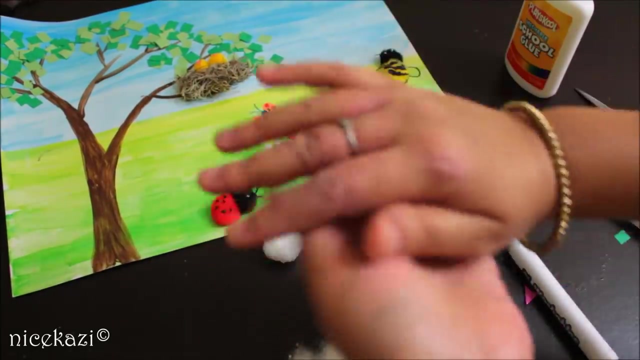 Now I am going to make a bumblebee with these pom-poms. Now, let's make a butterfly with this construction paper. Now, let's make a butterfly with these pom-poms. I used cotton for making clouds. Now let's make a butterfly with these pom-poms.